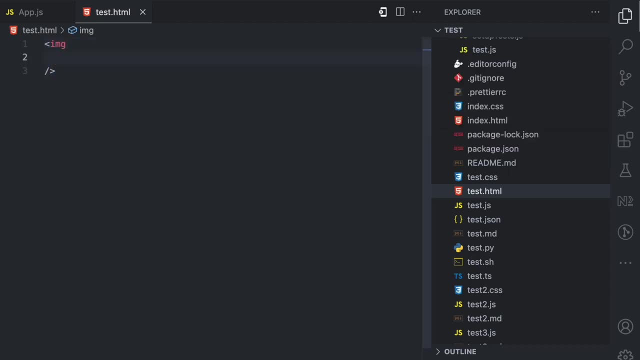 the img element. This img element is used for adding images to your application and it accepts different attributes, which you can also call properties or props. One of those attributes is src, which is the source of that image. I'm just going to add this image of myself here. It can. 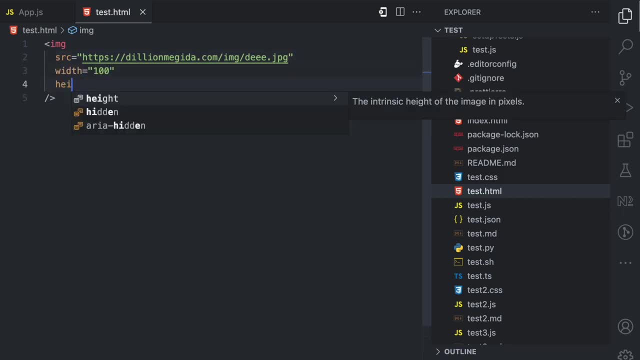 also accept a width property. Here we pass 100.. It can also accept a height property. We pass 100 again. It can also accept an id property, Of course a bunch of other properties, But before that, a bunch of elements in HTML can accept the id property as well as the class property or 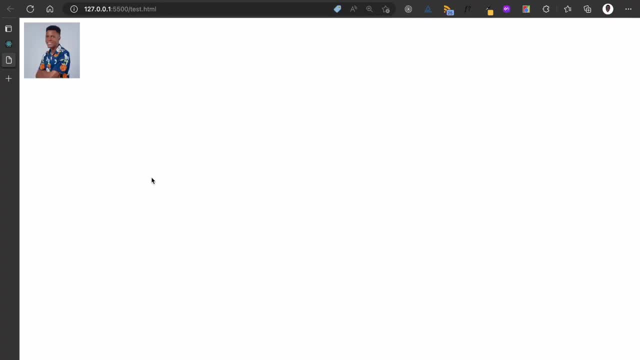 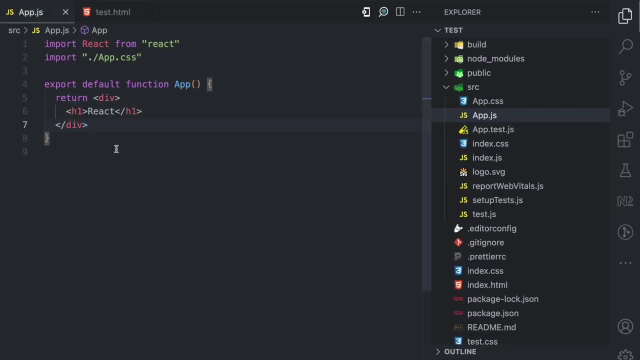 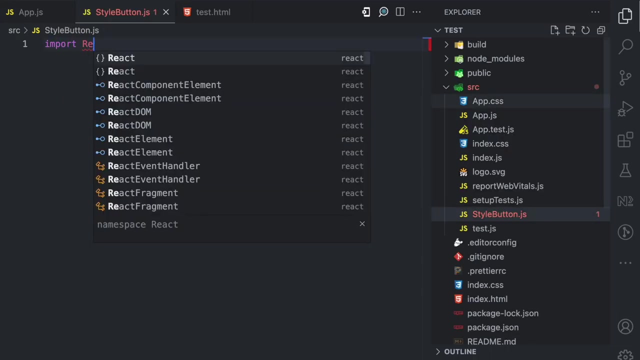 attributes And if we come here, this is the result on the screen. So the same way attributes apply to HTML elements is the same way props applies to components in React. So let's say I create a component here, I'm going to call this style button, Then I'm going to import React. 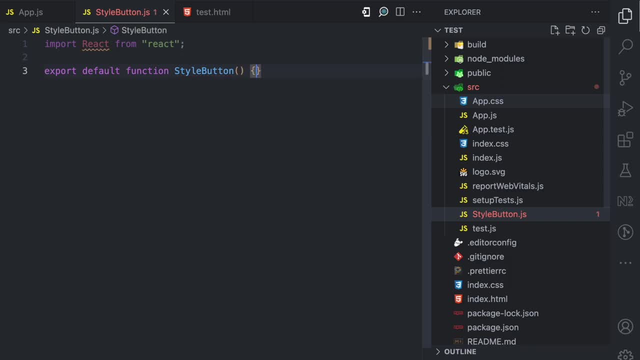 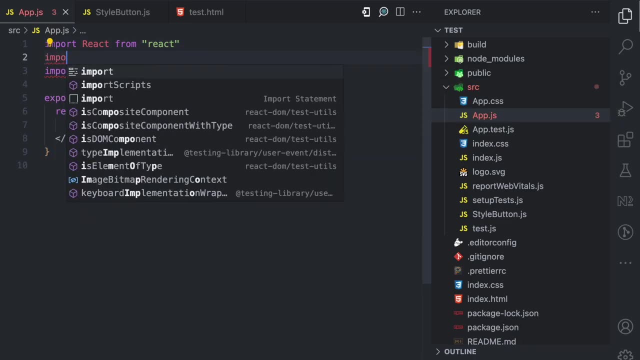 I'm going to export default style button And for now I'm just going to return a style button element. And then here in this appjs I'm going to import my newly created component style button, And I'm going to have style button here like this: Now we have this: 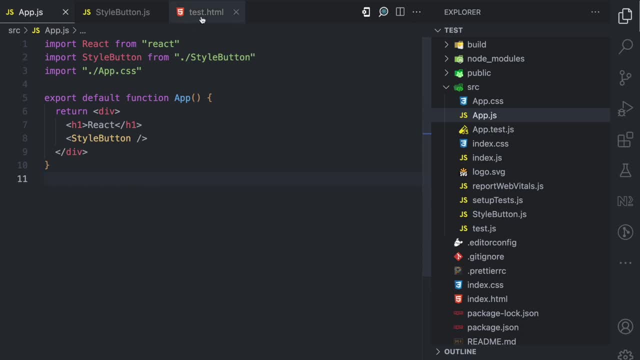 React component, and this component can accept props. just as we saw with this img element, We can also pass props to this component. So, for example, we can pass a label prop, And here I'm just going to add my name, Dillion. We can also pass a size prop, And in this size prop I'm just 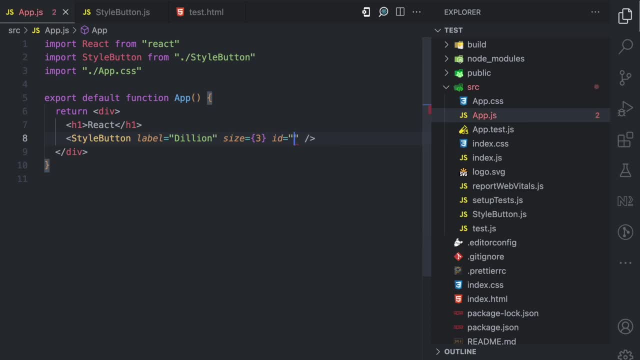 going to give it a number as three And we can also pass an id prop, And here I'm just going to say submit button. So for this React component style button we have passed three props, or you can say three attributes, which is label, size and id. I will come back to the screen And okay. 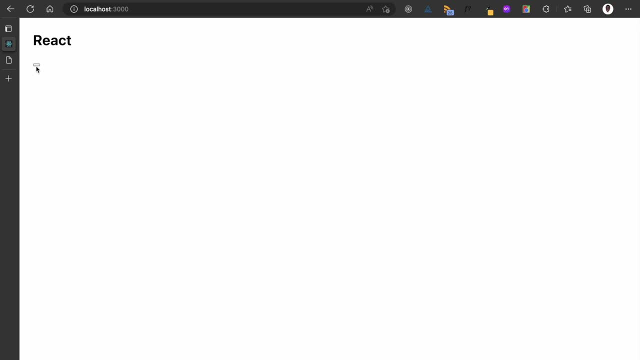 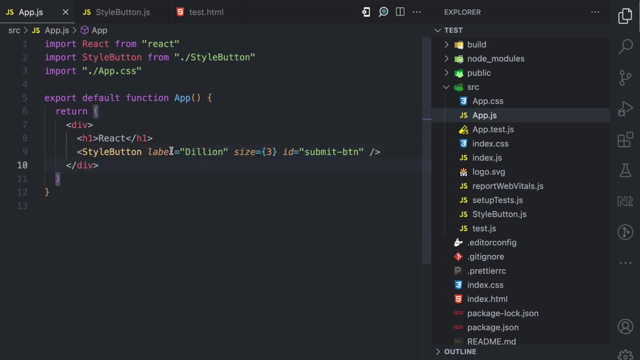 this is the one for the React app. If we refresh, you can see this is a tiny button here, But we are not showing the label, we are not doing anything with the size, we're not doing anything with the id. So, even though we are passing this as props to the style button component, we have not yet. 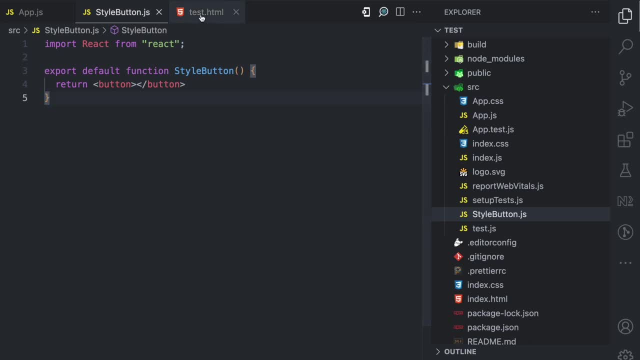 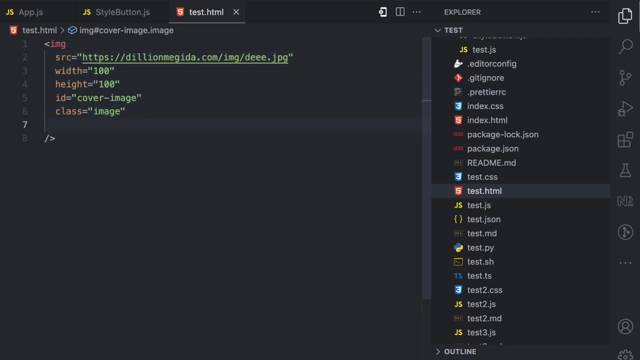 passed anything to the property. So let's say we pass props to the style button component. what props to expect? for example, when we come back here we know that the IMG element expects these props. let's say we pass a prop that this IMG element does not expect. let's say we pass a. 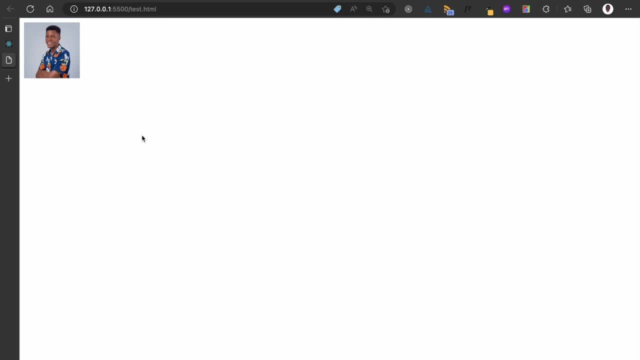 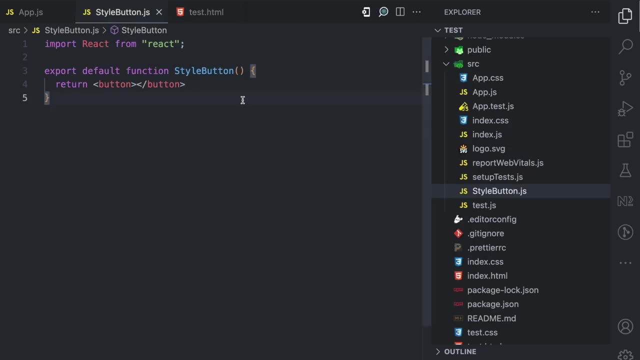 decode prop. And here we say decode. if we come back here and we check here, you can see the IMG element does nothing with that prop because even though you passed it as a property, it didn't expect it. So how do you define in this component what props to expect? Well, whatever props you pass, 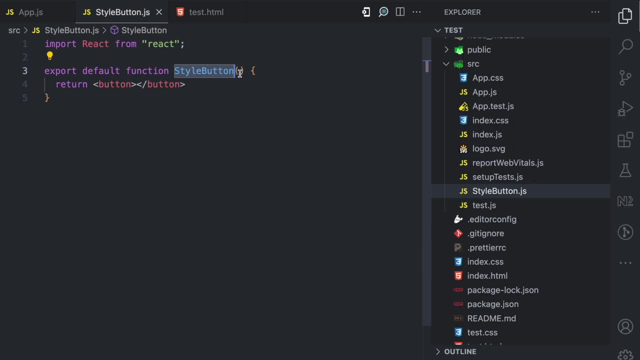 will be available as an argument to this style button function component. So you can give a parameter here called props. this is what people usually call it, but you can call it whatever you like. So when you pass props to this component, it will be available on this argument. So here. 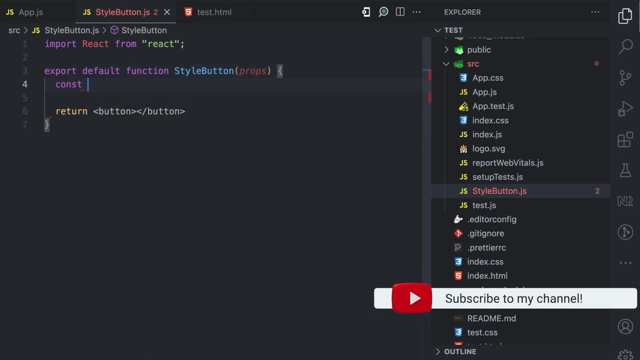 we can specify what props we're interested in. So we can say we are interested in the label property. we can also say we're interested in the ID property. we can also say we're interested in the size property, But for this example I'm going to act like one of these props, So we're going to 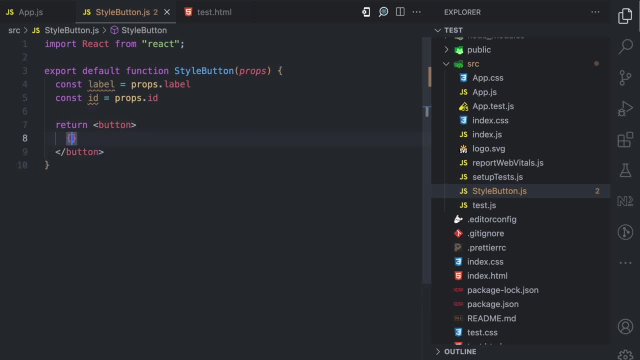 say we are not interested in that property. So here in the button I can place the label prop And for the ID I can say button ID and then I can pass this ID that comes from the props. So now we have been able to define what we expect for this style button component. So when we go back here, 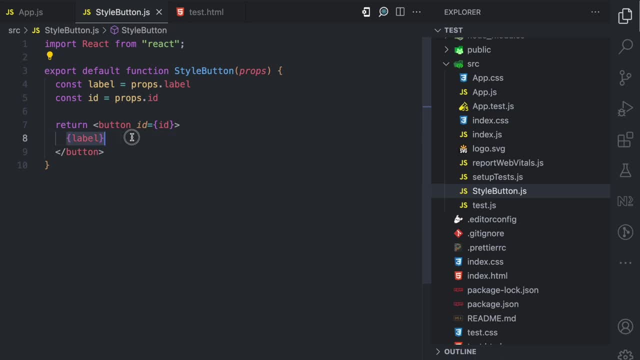 now and we pass this label, prop of Dillion, that means Dillion is going to be here when we pass this size of three. this component does not expect it, So it's not going to do anything with that prop. And when we pass this ID of submit button. 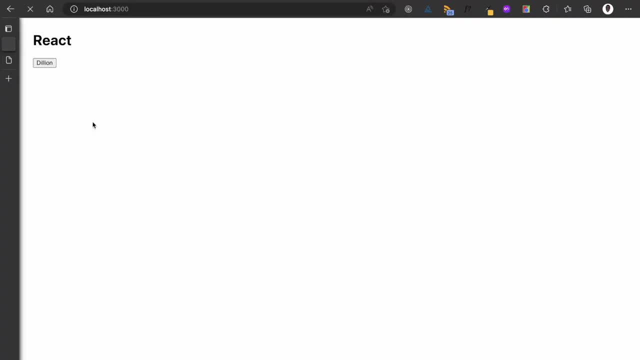 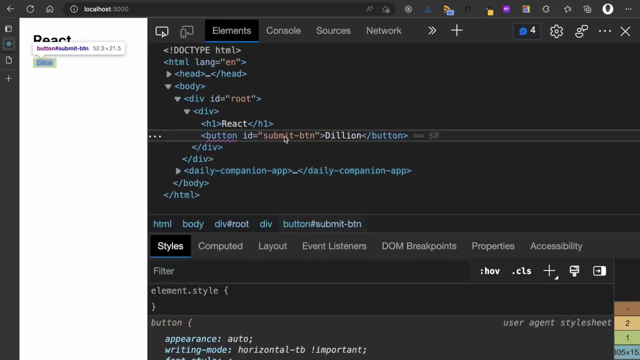 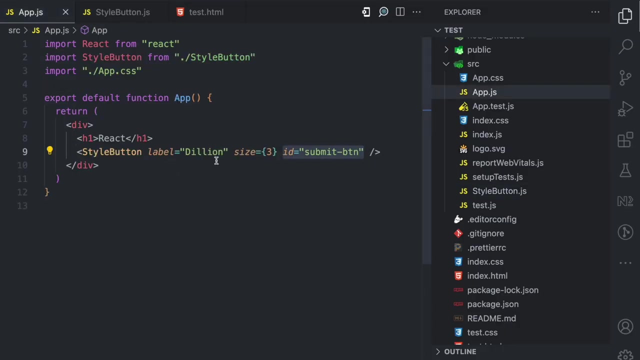 so that this component actually expects that prop. we go back here and refresh. you can see Dillion And if I inspect it, let me zoom in here. you can see the ID is submit button because we actually do something with the ID. So props can be of any data type. it can be a string, as we see. 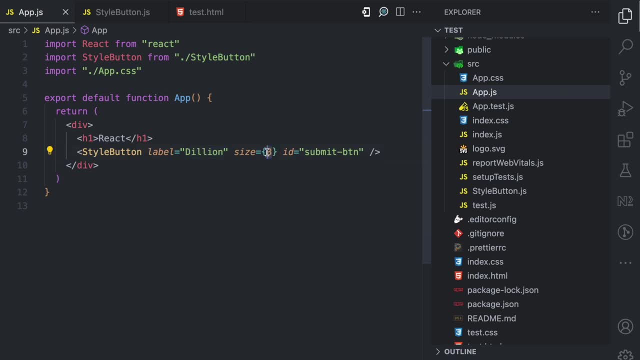 here. it can be a number, as we see. it can also be an array, it can also be an object. But one more example of a prop I want to show you is a function prop. So let's say we have a function here which.